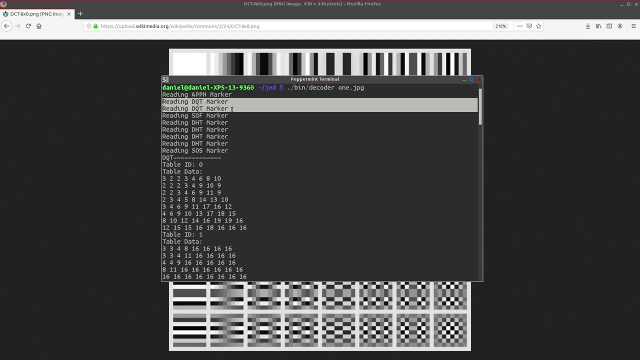 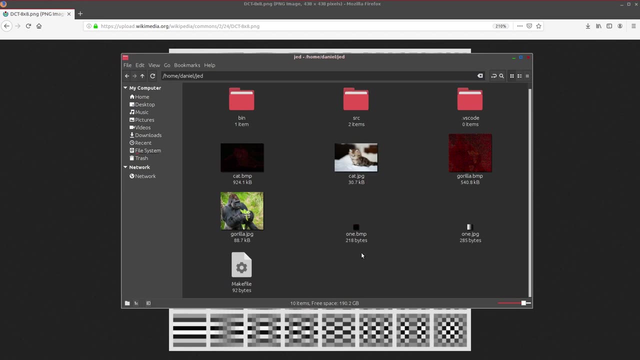 with an APPN marker, followed by both the quantization tables, the start of frame, four Huffman tables and the start of scan. So a very straightforward JPEG file. So here is one dot JPEG and here is the corresponding one dot BMP. Let's take a. 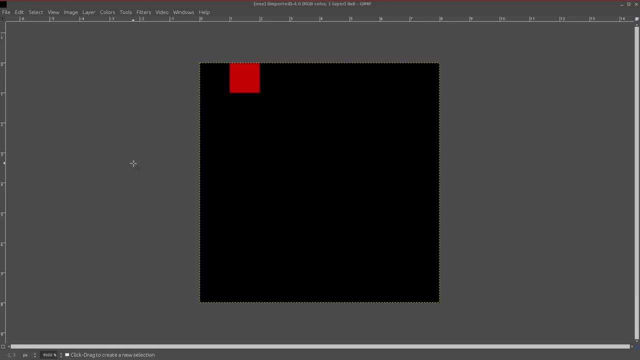 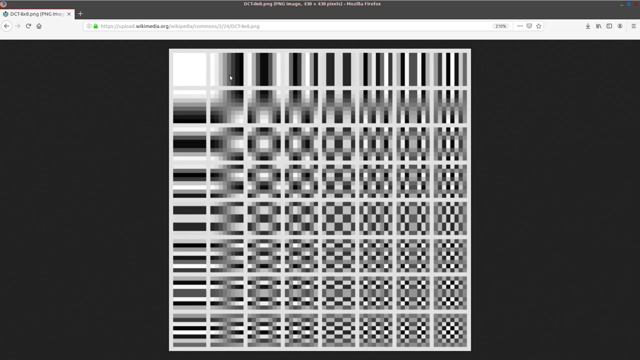 closer look. So here is one dot BMP and what we're seeing is the entire MCU is black or zero, except for one pixel which corresponds to the position of the image that we started with in this image here- and remember that the red comes from the luminance- 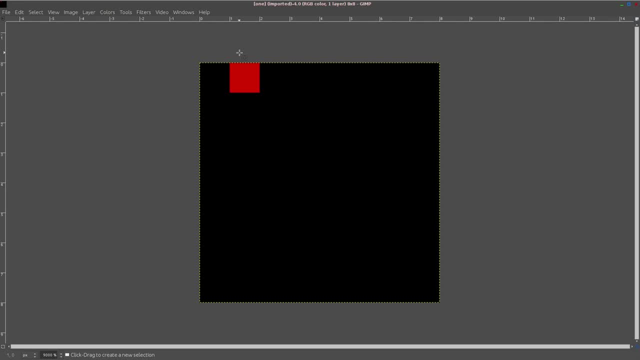 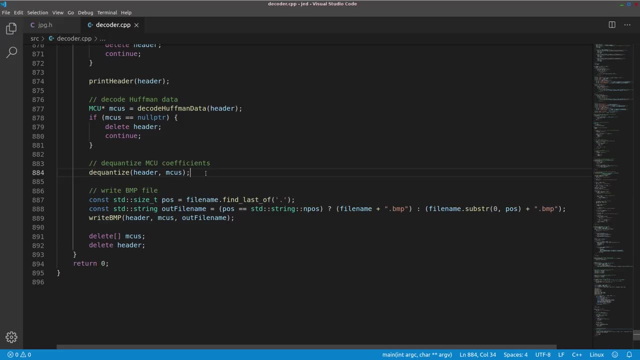 this is our volant dimers, and the white ones, are asked, are zero because there is no chrominance in the original image. but I think things will make even more sense if we are looking at the actual numbers. So here, after we de quantize, let's 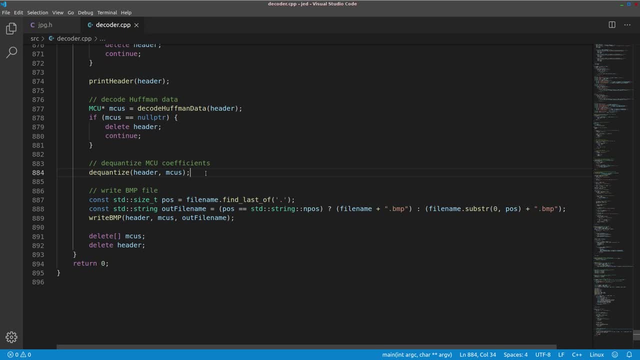 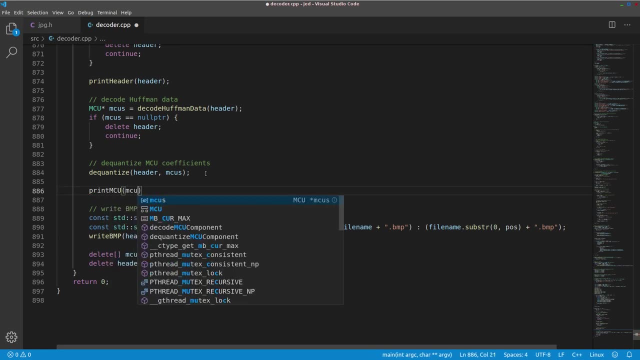 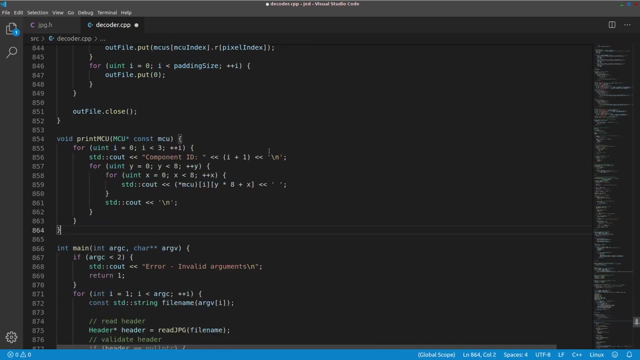 just print the content of the MCU. That way we can see the actual DCT coefficients, amo, nd. let's just throw that in write-down image: The actual Cor합 tr nd, ru, p, ut here. This code is really not important because it's very temporary. We just want. 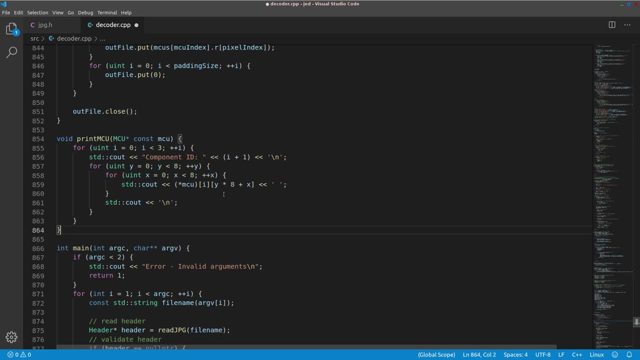 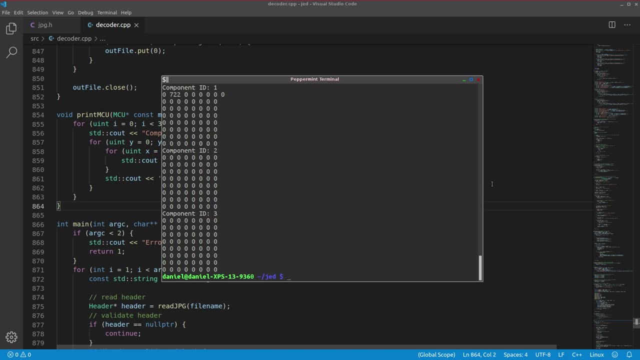 to print all 64 values in the first MCU of the image, And this does match our predictions. The coefficients for both of the chrominance channels are all zero and all but one coefficient for the luminance channel is zero. Now remember that the first coefficient, the DC coefficient, represents the overall 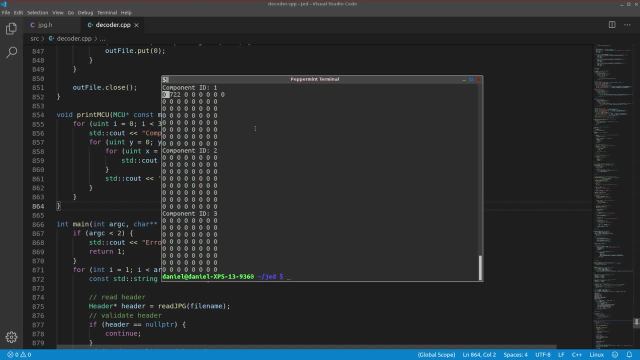 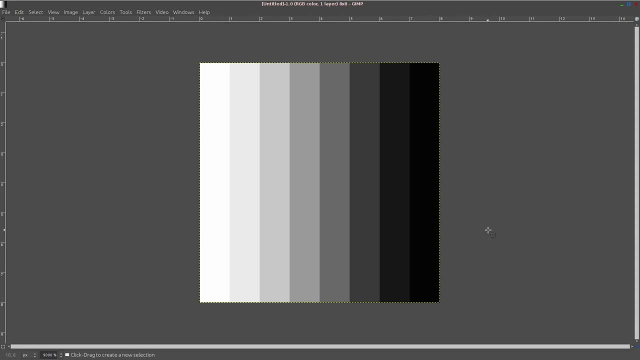 brightness of the MCU. So it's kind of interesting there's a zero here. It kind of makes sense If you think about the average brightness of all of these pixels. we have some in the middle that are a middle gray and we have both extremes with bright white and dark black on the sides. So it all averages. 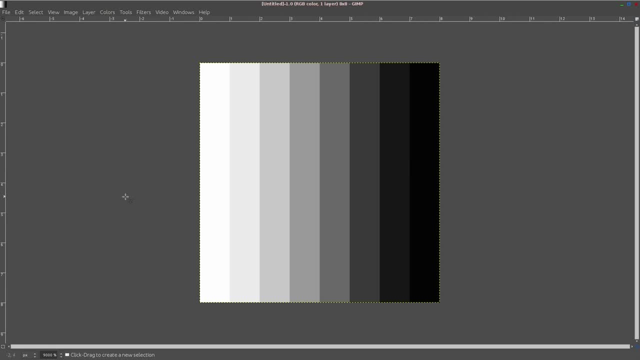 out. So the average brightness is about middle gray. So what we learned is that a- an average brightness is about a middle gray. So what we learned is that a middle gray is about a middle gray. So what we learned is that a- A DC coefficient of 0 means the average brightness. 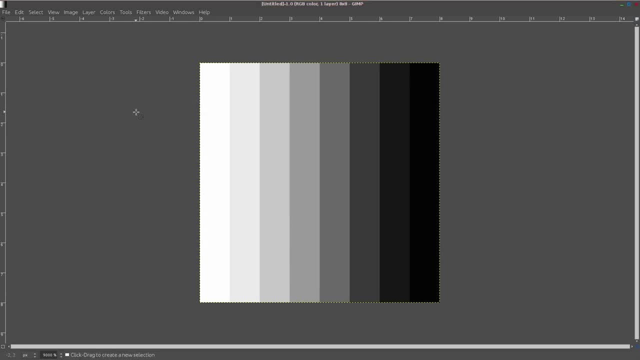 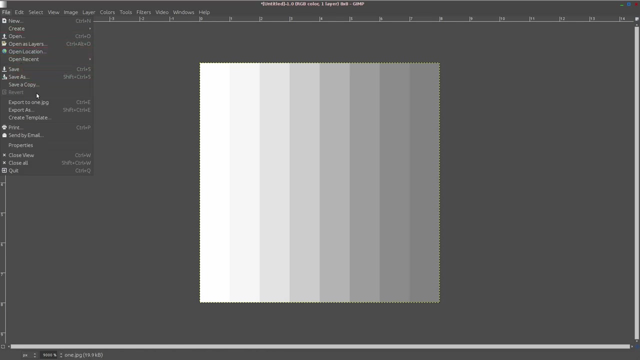 is medium brightness, Hopefully. what that means is we can increase or decrease the brightness of this image and we will see that reflected in the DC coefficient. So let's go ahead and crank up the brightness and overwrite 1.jpg Now. if we run this again now, we 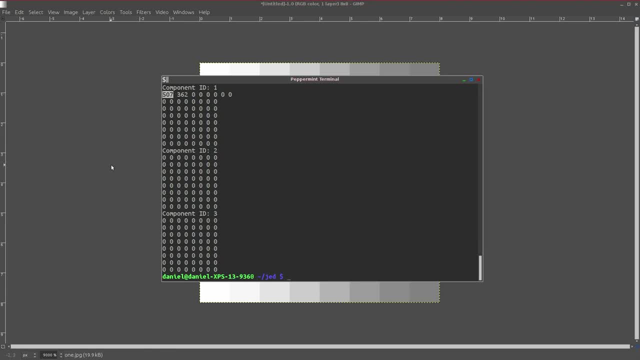 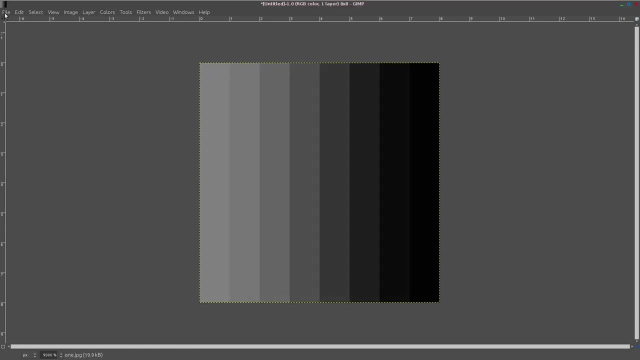 see a very large number as the DC coefficient, indicating that the MCU is very bright. As far as the image pattern goes, this is still the only non-zero coefficient, because the image data is perfectly explained by this one pattern. Likewise, we can decrease the brightness and overwrite 1.jpg. 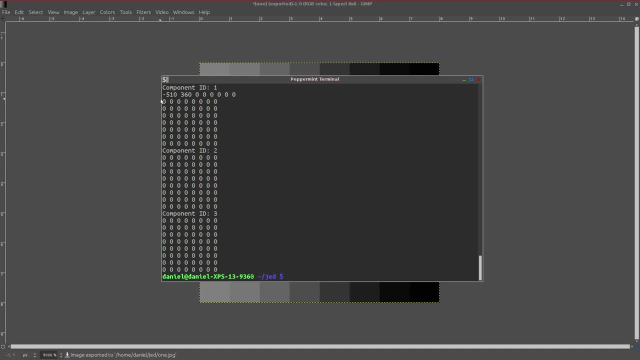 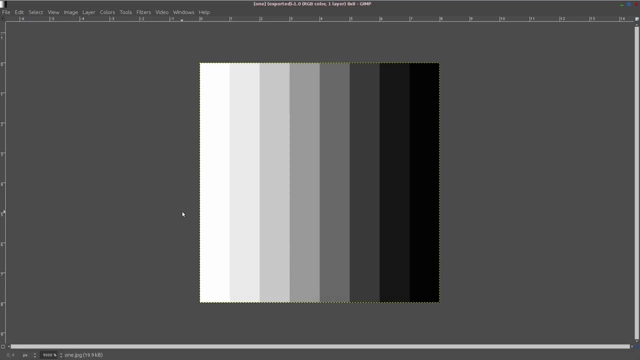 Now, when we rerun this, we see a very large negative number, as the DC coefficient indicating the MCU is very dark, and again only one non-zero AC coefficient. Here's one more important thing to point out about how these image patterns work. 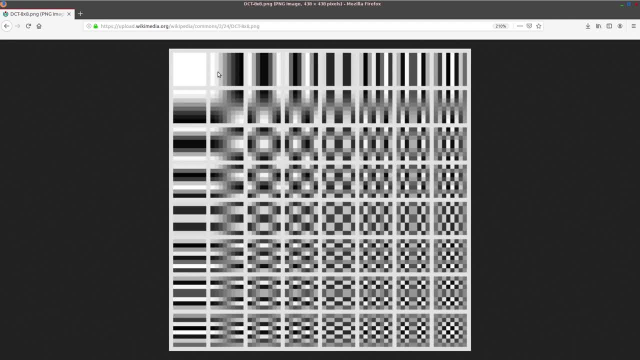 We see this image here, with all vertical stripes of a single color, with white on the left and black on the right, But none of these 64 images show vertical stripes with black on the left and white on the right. So what if that is what our image looked like? 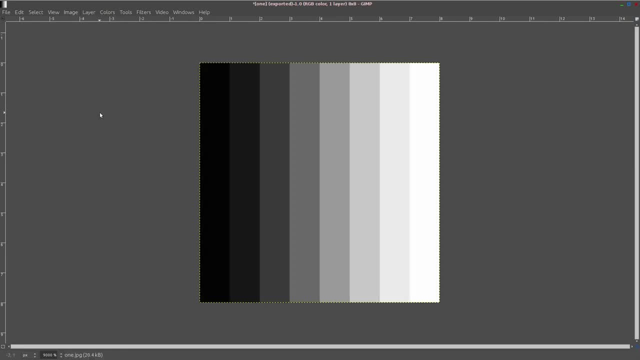 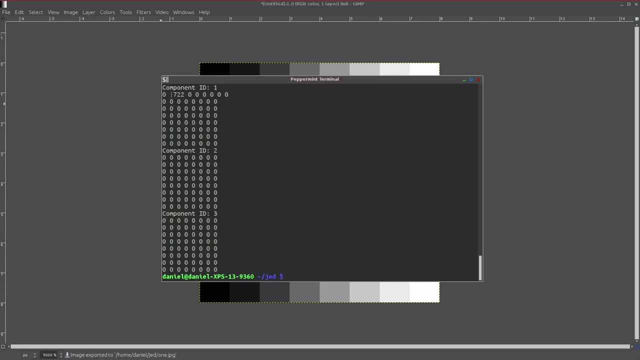 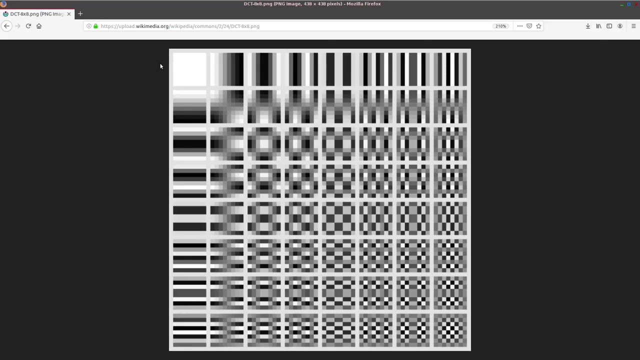 Here we can flip the image so that the black is on the left and overwrite 1.jpg. And now we have a very large negative number for that same AC coefficient. So here, with respect to the DC coefficient, a positive number means an overall lighter MCU. 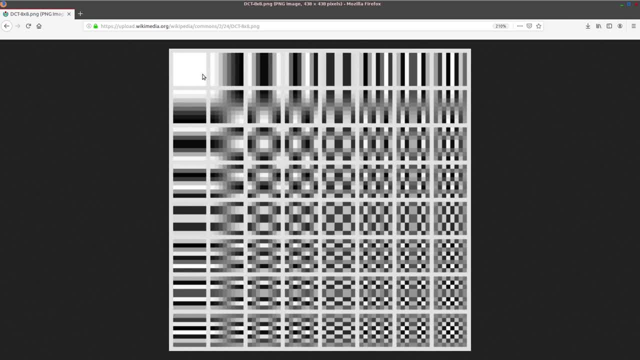 and a negative number means an overall darker MCU. But with the AC coefficients a positive number means a positive contribution or a direct contribution and a negative number means a negative or inverted contribution. Knowing all of that, knowing that we can control the brightness and use. 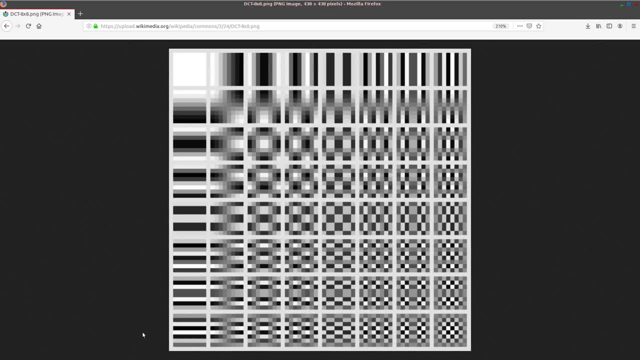 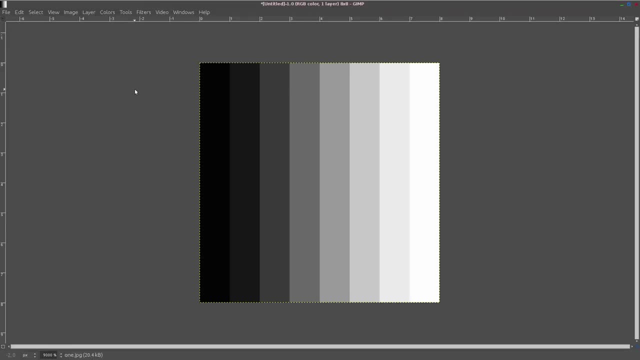 any combination of the other 63 images, along with their inverse. we can use all of this information to create any possible. So let's take a look at an 8x8 MCU that we want. So here's the real question. Let's go back to our first image we started with. 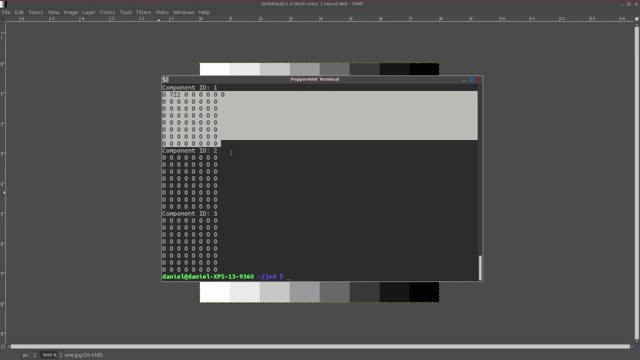 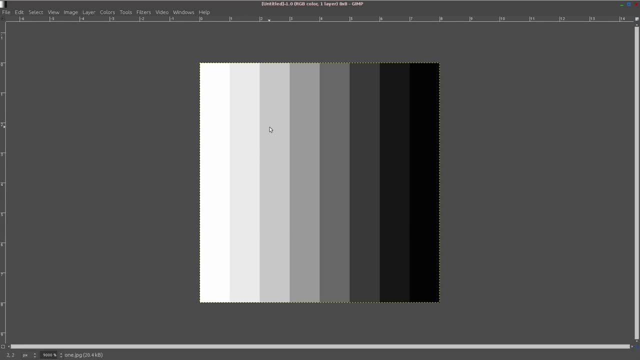 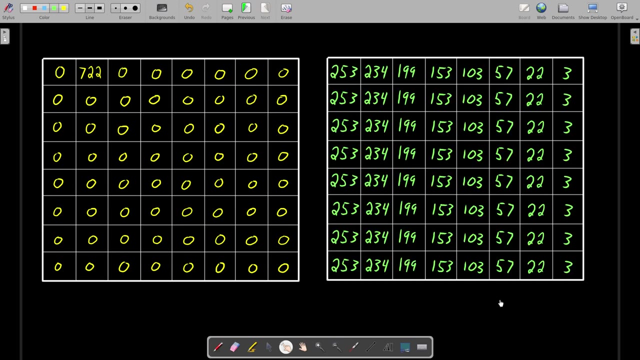 Here is the luminance data for the MCU in terms of discrete cosine transform coefficients. How do we convert this to an MCU with the correct luminance data for all eight of these columns? In other words, how do we transform this matrix into this matrix? 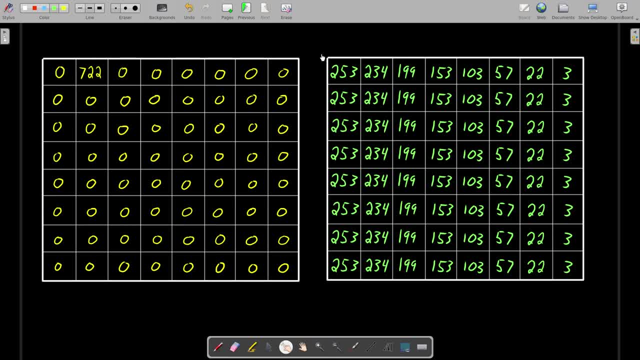 With just this one piece of information, we need to be able to fill each of these columns with the correct color. Now we really get into why cosine? Why is cosine a part of this process at all? Let's hone in on the image that corresponds. 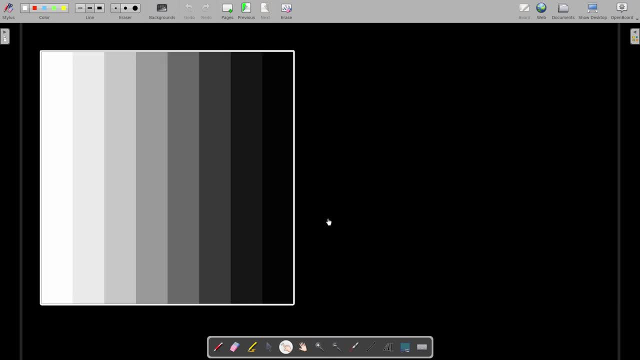 to this DCT coefficient. So here is that image again. Let's make a plot where we graph The x position or the column number on the x-axis And on the y-axis let's graph the column's color, where white is 1, black is negative 1, and middle gray is 0.. 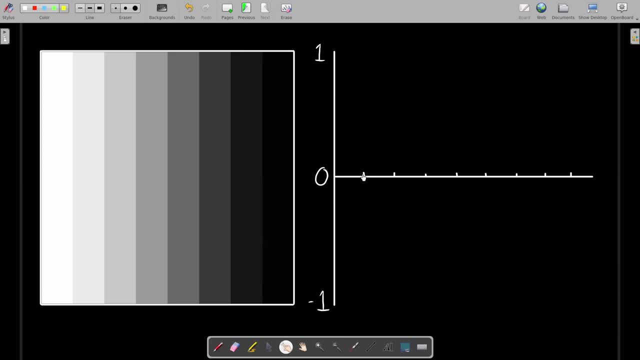 So if we plot this near perfect white, that will be basically at 1.. This next column will be about here. The third column will be about here. As we get to the fourth and fifth column, we get very close to middle gray. 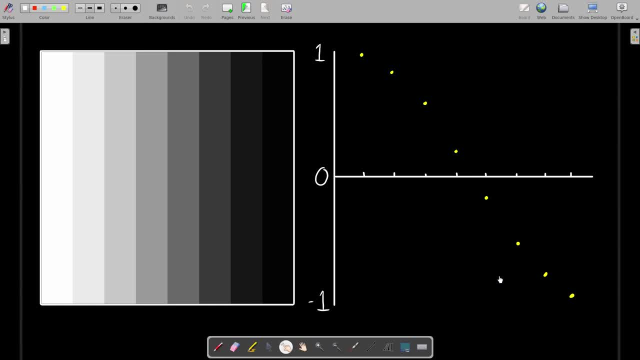 And I'll go ahead and plot the last four Now. my crude drawing isn't perfect, but this gives you a pretty good idea of how it's supposed to look, And you might notice that this isn't exactly linear. In other words, the delta from column to column. 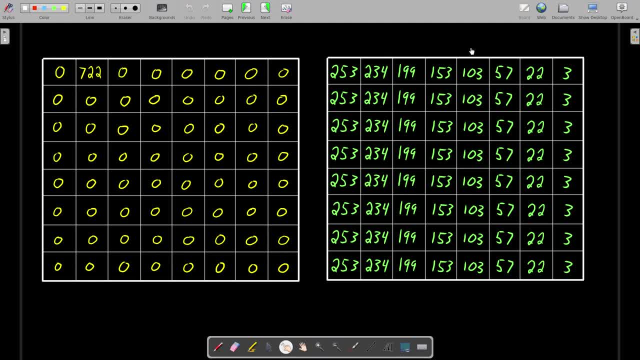 or how much it decreases by, is not a constant amount. Between column 4 and 5, the value decreases by 50. But on the edges here and here it only decreases by about 20.. So if we connect the dots, 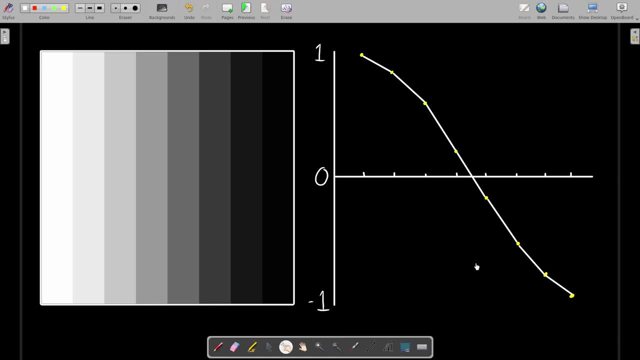 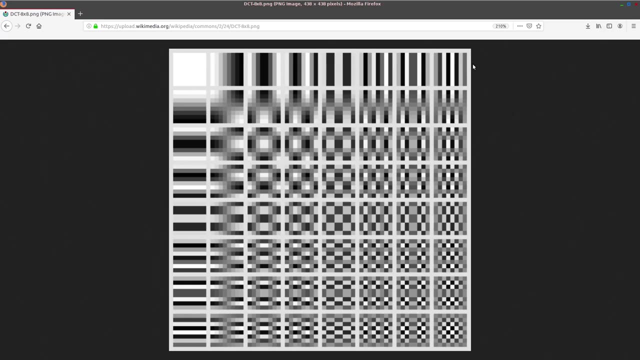 you can see, this looks a lot like part of a cosine graph, And that's exactly the idea. The idea is that this is a cosine graph with a very low frequency. It takes a long time to transition from white to black, Compared to this image here, which 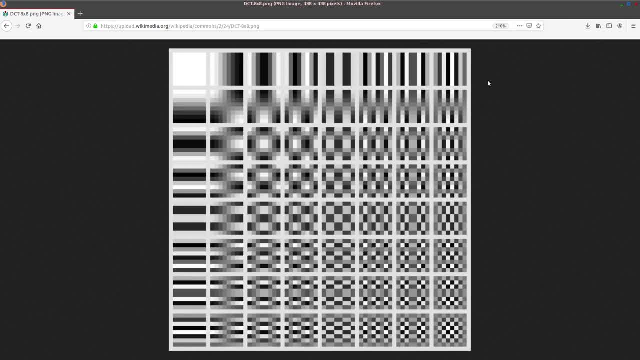 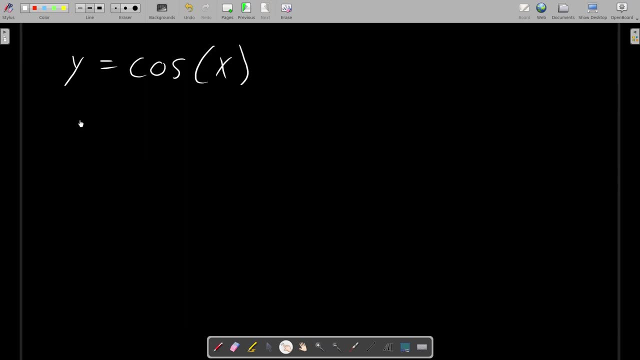 represents a cosine wave with a much higher frequency. It oscillates back and forth between white and black many times within a single MCU. So what do we know about the equation of a cosine? Well, in the most basic form we know: y equals cosine of x. 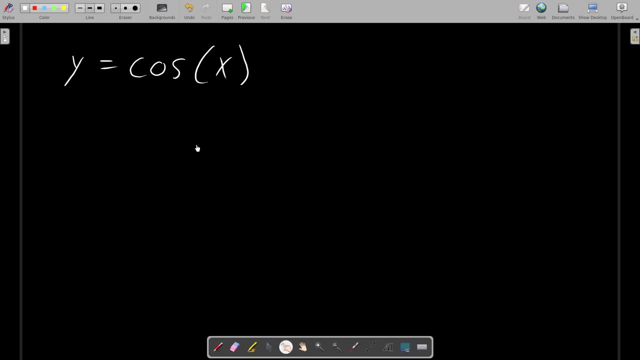 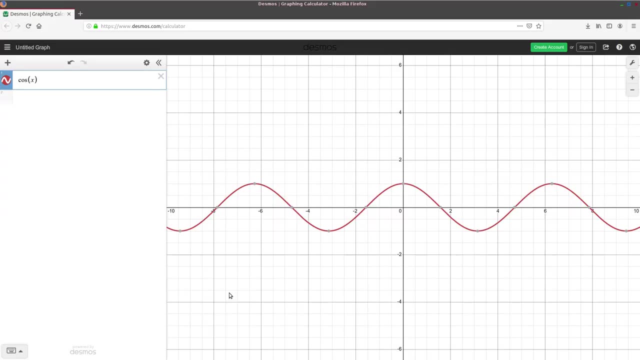 We'll give us a simple cosine wave that oscillates from 1 to negative 1.. That's just the basic cosine. But how can we modify this equation? Here's a basic graph of y equals cosine of x. So what can we do to modify or parameterize this equation? 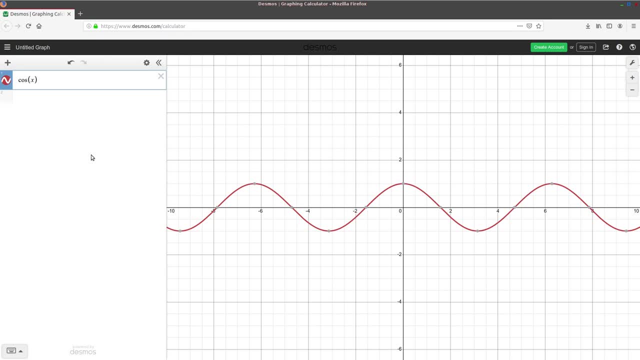 One thing we can do is multiply the entire equation by some constant which changes the amplitude of the wave. We can change this constant to 0, which flattens the entire cosine wave into a straight line. This constant that we multiply, we multiply by, is like the DCT coefficient in our MCU. 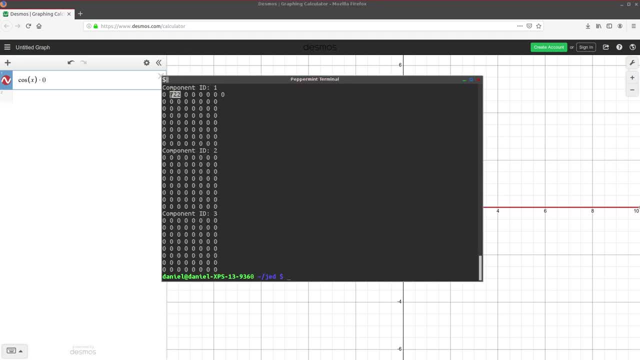 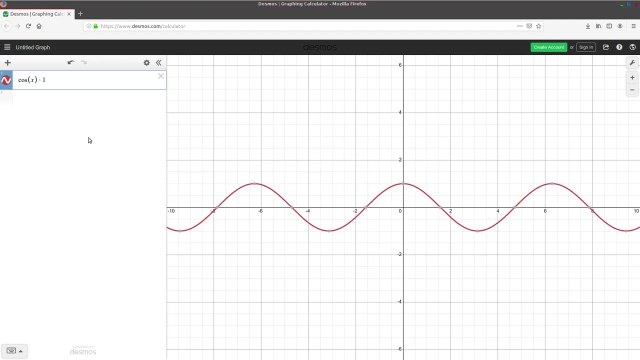 This is saying that the cosine wave that corresponds to this location has an amplitude, essentially of 722.. And the amplitude of every other cosine wave is 0.. In other words, they do not contribute to the image. This should also show why negative numbers 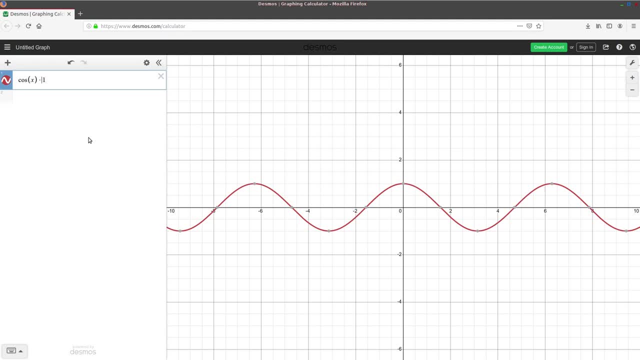 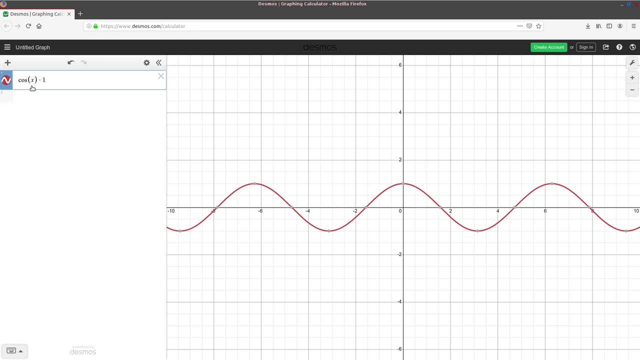 If we multiply the coefficient by 0, we'll get 0. x by some coefficient to control the frequency of the wave. As we double this coefficient, we double the frequency. Now, if this coefficient here is like our DCT coefficients in the MCU, this coefficient here is like the x and y position of 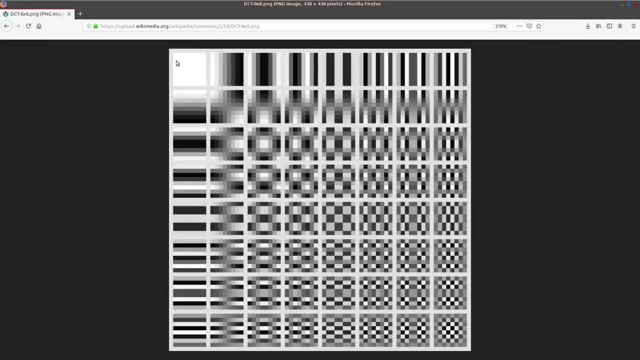 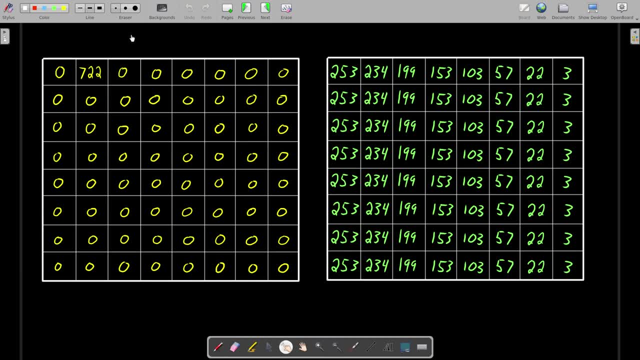 each coefficient in the MCU, Larger x values correspond to higher frequencies. So how do we use this DCT coefficient data to calculate this color data? Well, for every one of the pixel values that we want to calculate, for all 64 of them, 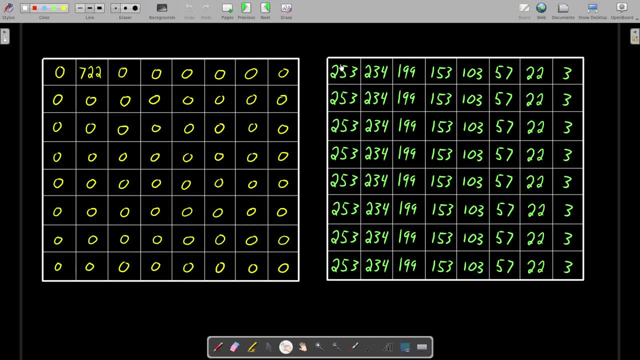 its value is the sum of the contributions of 64 cosine waves. So you can guess that's going to be quite a bit of computation. For all 64 positions we need to sum 64 cosine waves. There will be some optimizations. There will be some optimizations. There will be some. 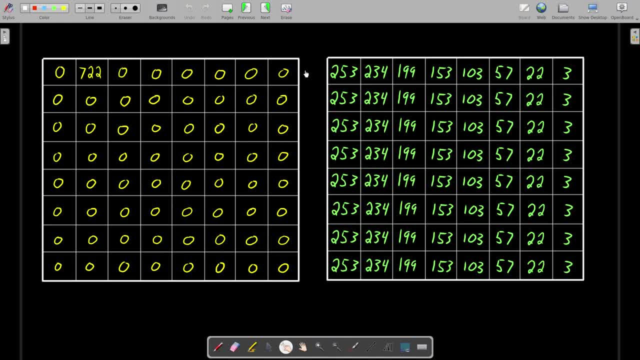 optimizations that we can end up doing. that we'll discuss in a little bit. Because all of these coefficients are 0 aside from one of them, our summation will end up being this: one cosine wave plus 63 other cosine waves that all have an amplitude of 0.. For now, 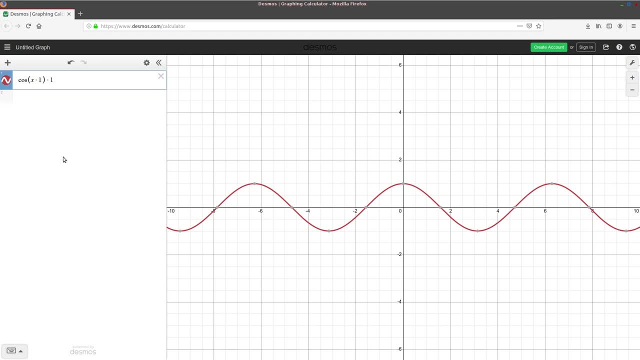 let's see what happens when we sum two cosine waves instead of 64. When we sum two identical cosine waves, all that does is we sum the two cosine waves. So we have 64 cosine waves. we sum 64 plus 3 quasi clamples, we sum 64 main shear and we sum 65 도 as well. And 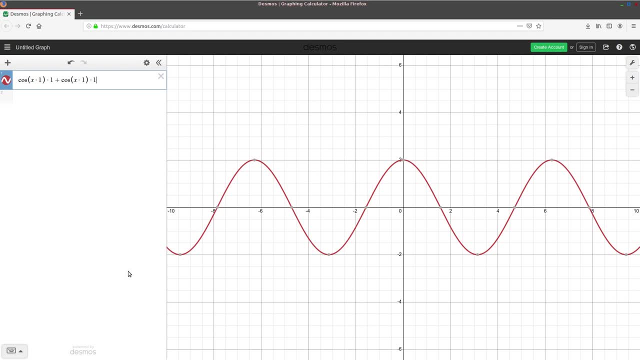 now what we're really going to do is we specifically assign the formula of come in eigenvalues. what value that gives us? We'll use that instead of the function count. So come in eigenvalues. what we're going to do is we're going to add the 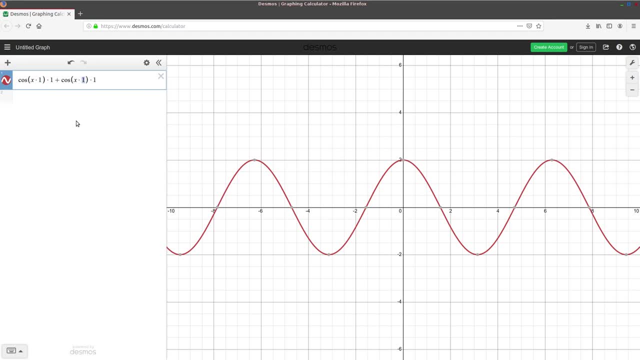 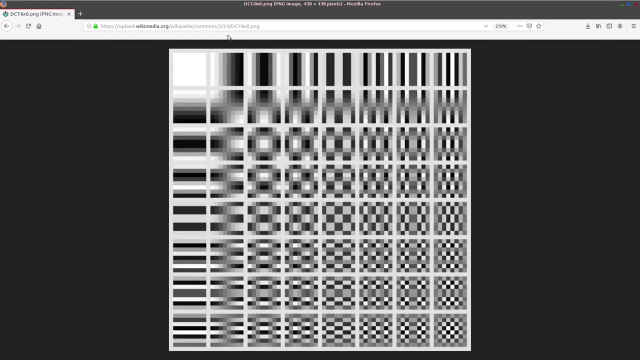 convention sum as the function count. So it has the function UN. come in Now using a definition that's not exactly real. example can be a little in the actual calculations, but the effect is the same over here. So let's say we're summing the. 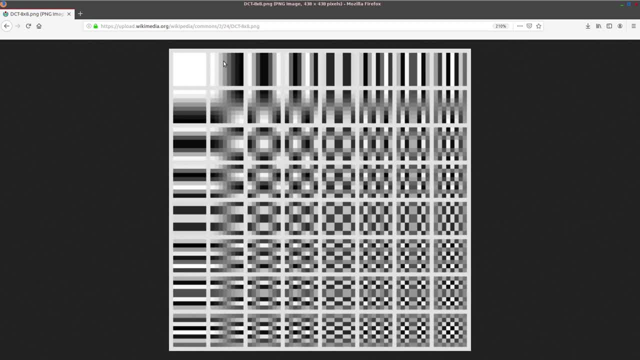 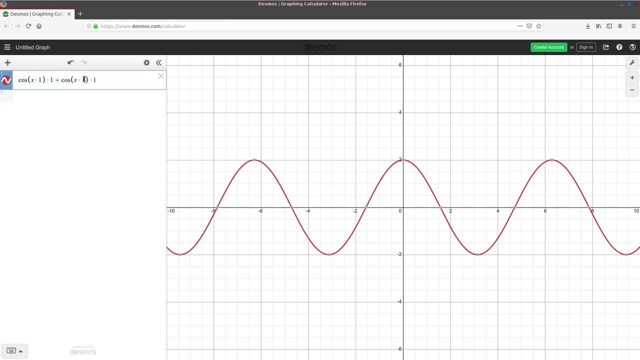 cosine wave for some cosine with a lower frequency and adding that to the cosine wave which has a higher frequency. So if we add two cosine waves, one which has four times the frequency as the other, this is the resulting graph, at least whenever the weights of the two waves are equal. 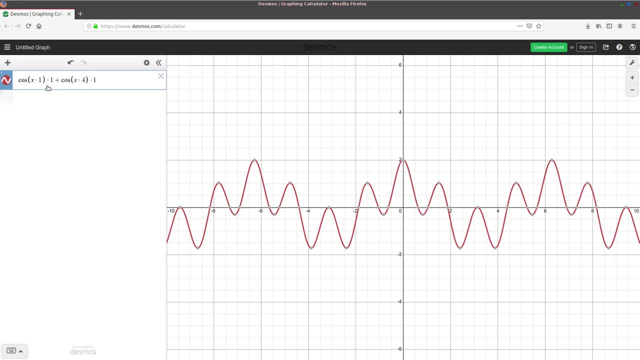 What if we say the weight of the first wave is 10 times greater than the weight of the second? We can also make one of these weights negative. You can already see how this produces pretty complex waves. and we're only adding two, not even close to the full 64.. So now what we really need. 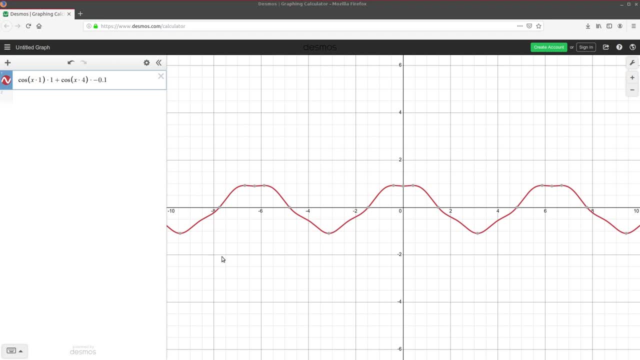 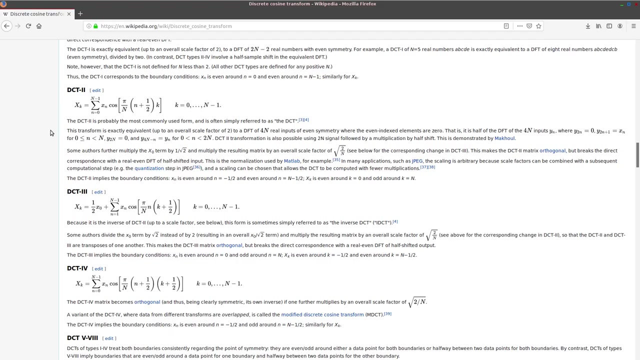 is the summation formula that tells us exactly how to sum all 64 cosine functions, given their amplitude, the actual DCT coefficient and given the x and y position in the MCU, or in other words the frequency of the wave. For that we can turn to good old Wikipedia Here on the page all about. 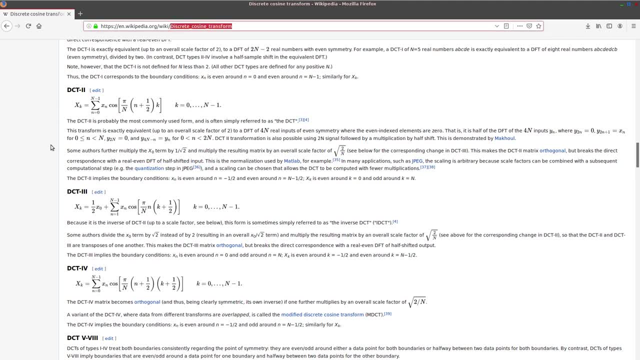 the discrete cosine transform. there are many examples. The primary one, used by JPEG compression or JPEG encoding, is DCT number two, and DCT number three is the inverse of DCT number two. So DCT number three is the one that we need. However, this 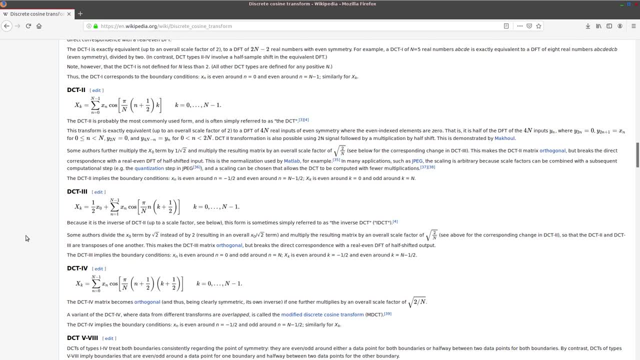 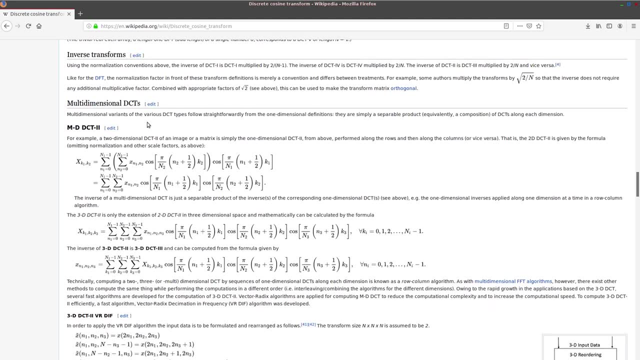 explanation. here is a one-dimensional DCT. We need a two-dimensional DCT. Wikipedia has this whole section on multi-dimensional DCTs. Here they show the 2D example of DCT number two, which is not the one we're using right now. You know it's 2D because 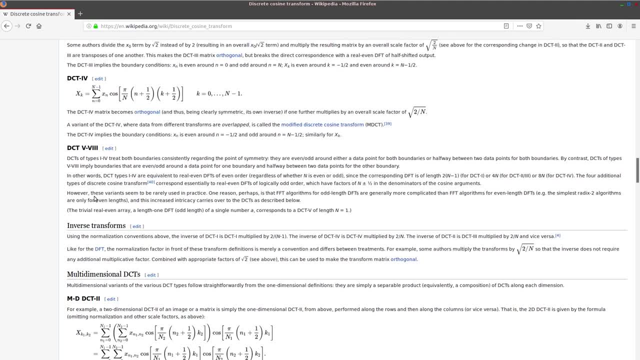 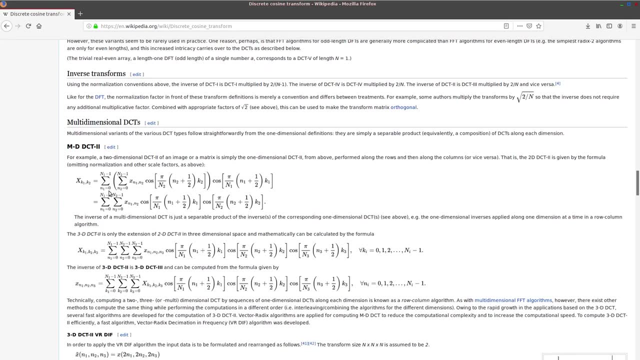 there are exactly two summations, However. this goes from the 1D DCT number two to the 2D DCT number two. This is the same change we have to make to go from the 1D to the 2D DCT number two. 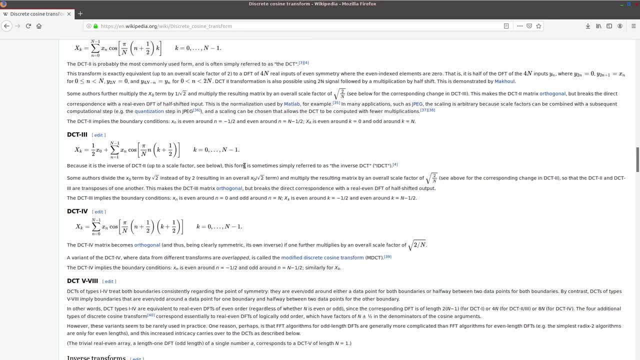 DCT number 3 to the 2d DCT number 3, which is not shown here on Wikipedia plus, there are more details about how JPEG specifically uses DCT, like some additional factors and other things that play into the calculation that are not shown here. but I think this video is going to be long enough even without 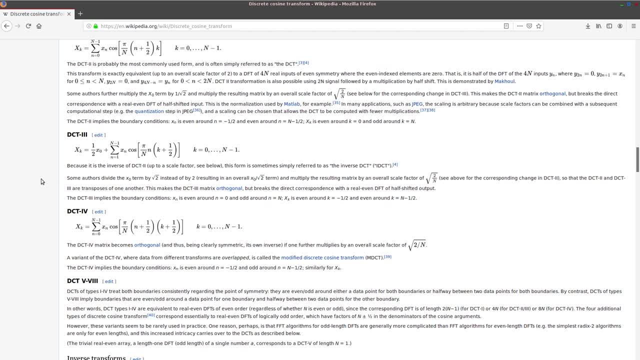 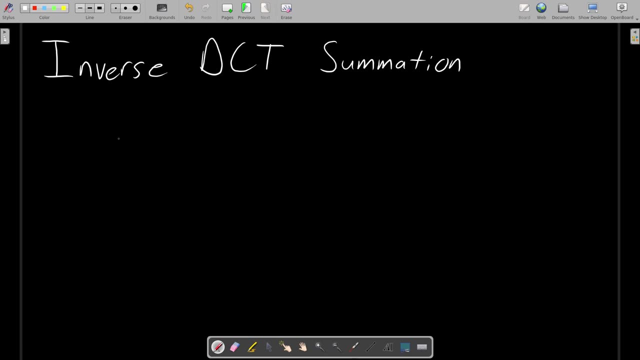 dissecting this summation. so if you want to dissect it, feel free. but I'm going to cut to the chase a little bit about how we need to use it. so let's start by writing the summation algorithm in a little bit of pseudocode. I already 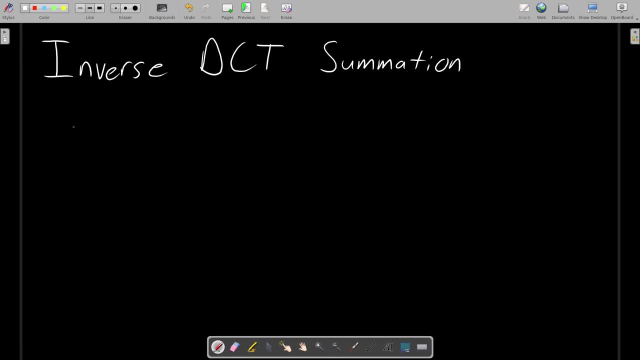 implied that we need to loop through every pixel. so you can assume there will be some nested for loop for Y and X. so for Y and X going from 0 to 8, inside this nested for loop, we will calculate the color. for Y and X going from 0 to 8, inside this nested for loop, we will calculate the color for. 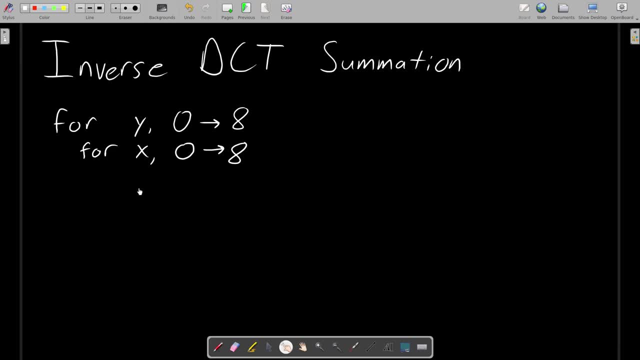 one pixel, pixel XY. to do that, we have to sum all 64 cosine functions, so let's initialize sum to 0. now we need another nested for loop. since we're already using Y and X, let's just call them I and J. so now we use I, J as the coordinates. 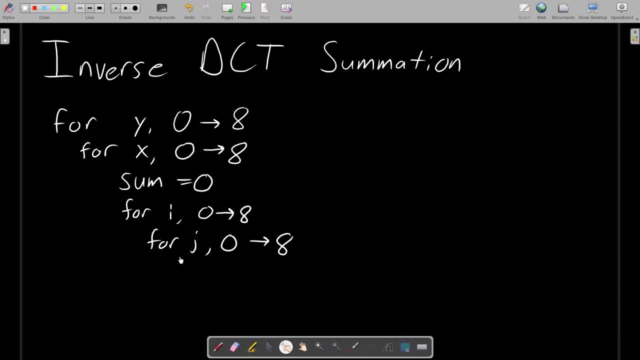 of a discrete cosine transform coefficient or a weight of one of the 64 cosines and we use that weight to scale some cosine function and then add that to our sum. but it's actually a little bit more complicated than that. this is the DC coefficient I- J. we also need to multiply this by two other. 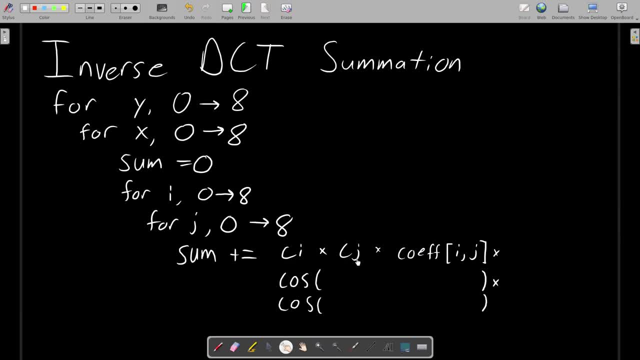 coefficients, one that depends on I and one that depends on J, but we'll talk about those in a little bit. and because this is a 2d DCT and not one D, we multiply this by two different cosine functions. so this here handles the amplitude or weight of the cosine, and whatever we need to put inside here will. 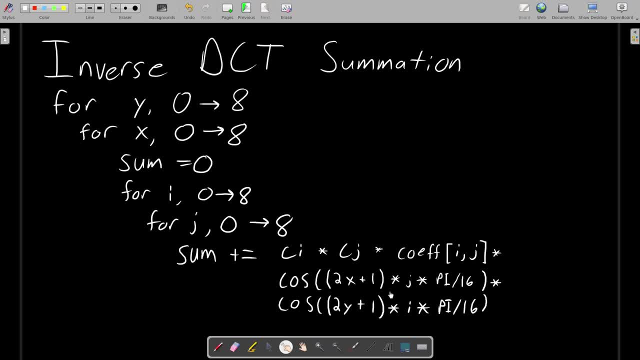 handle the frequency. so the two cosine functions that are included account for the two dimensions. so one of them uses X and J which, if you think about it, they kind of correspond to each other. X is the inner of this nested for loop and J is the inner of this nested for. 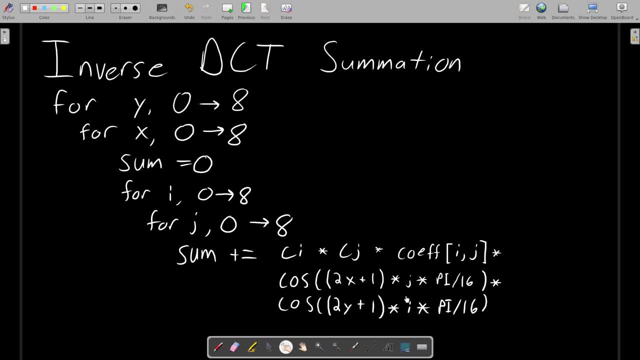 loop and the second cosine function is Y and I. the 2 multiplier and the plus 1, as well as the extra constant here, times PI over 16, are just part of the definition of the JPEG inverse DCT and I apologize, I'm kind of trying to fit too much on. 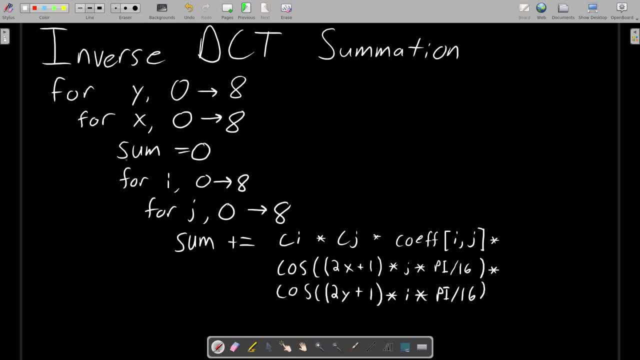 screen at a time, but the last part is after this nested for loop is finished. sum is divided by 4. after this, the value of sum is the pixel intensity for pixel XY. the only thing left is to talk about where CI and CJ come from. well, by default. 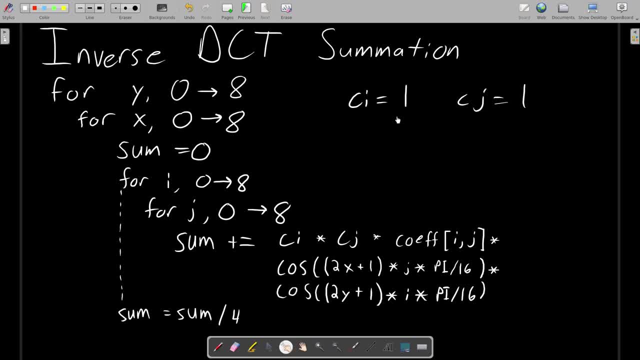 they're both equal to 1, but only in the case where I is equal to 0 instead, then CI equals 1 over the square root of 2, and same thing with CJ. if J is equal to 0, then CJ equals 1 over the square root of 2. 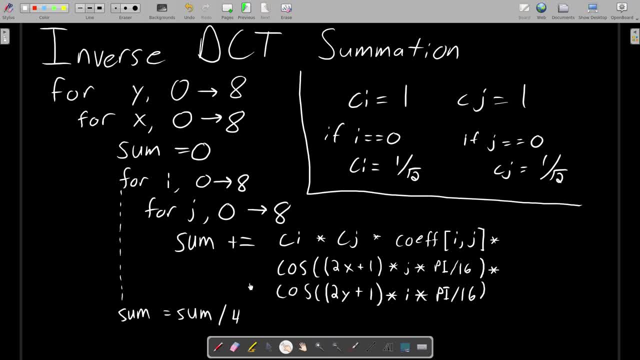 just one more really important thing to point out about how this has to be done. once we get the sum of all 64 cosines for a single cosine function, then we can pixel xy. we can't simply write the sum directly back to the MCU at position xy. 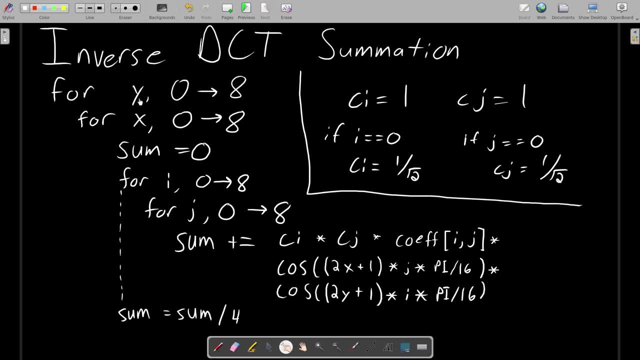 because for the rest of this nested for loop we will continue reading from our MCU. Basically, this array of DCT coefficients is our MCU component. That's where the DCT coefficients are stored. But we need to be able to read all 64 DCT coefficients for the entire duration of this nested for loop. So when we 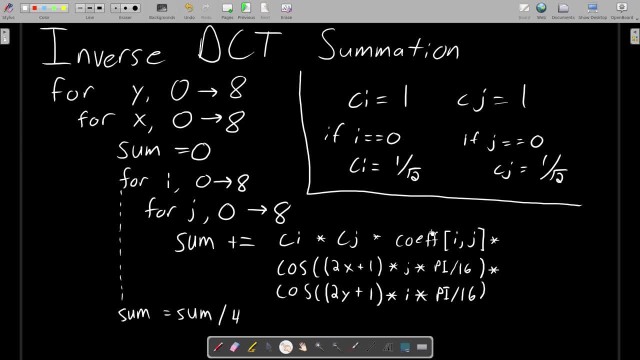 calculate a final sum, we cannot overwrite the corresponding DCT coefficient at xy. Otherwise we will be unable to correctly calculate all following pixels. So all that means is we have to store these resulting sums somewhere else. Then, when this is all said and done, we can copy all of the 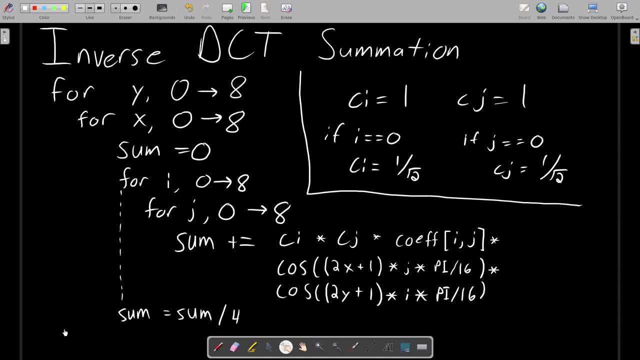 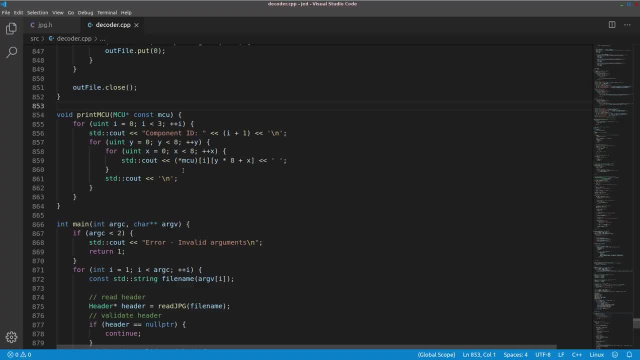 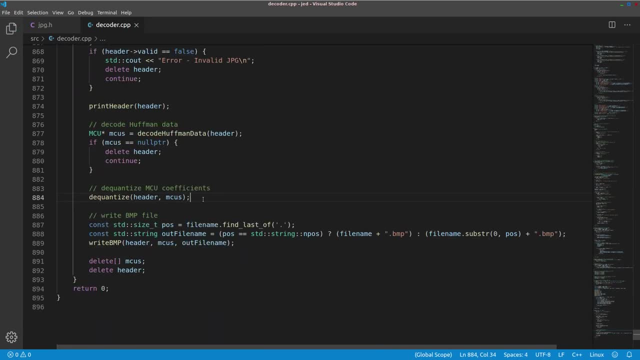 subway sums all of the color intensities back to our MCU component. Okay, so let's give this a shot and implement all of this in our decoder. Let's start by undoing this print MCU thing. After we de-quantize all the MCUs, we want to perform inverse DCT on all the MCUs. 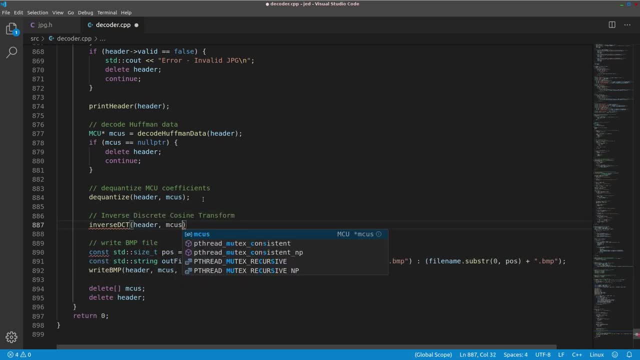 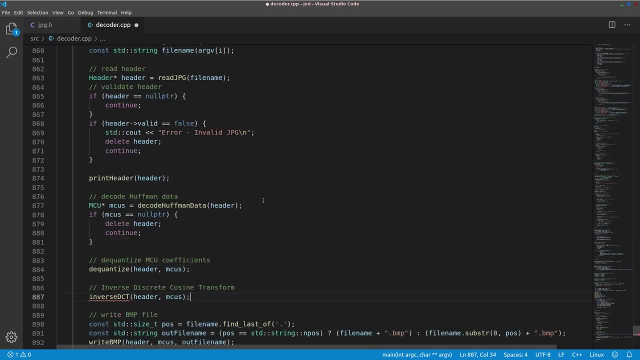 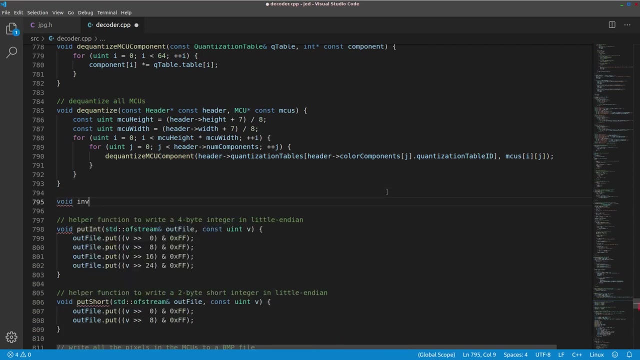 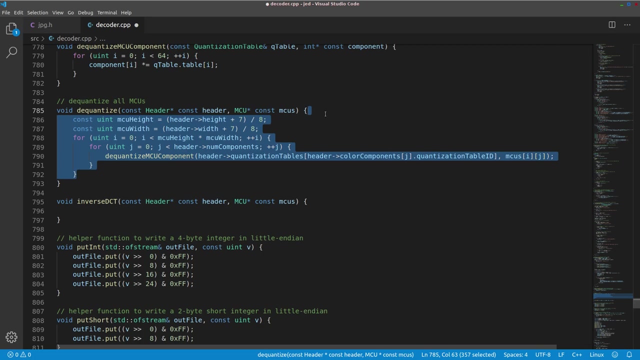 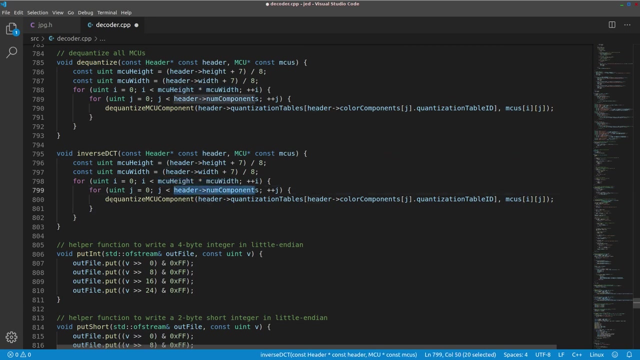 Then let's add this inverse DCT function below the de-quantize function. We're going to use the exact same pattern that we used for de-quantization, which is for every MCU and for every quantum. So we're going to add a component in that MCU. 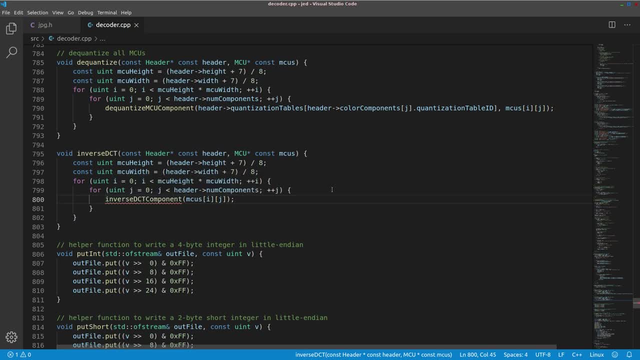 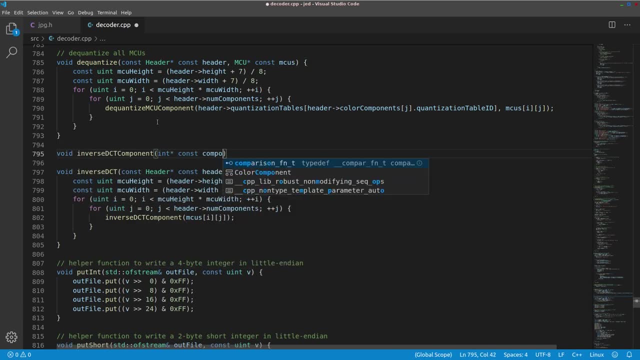 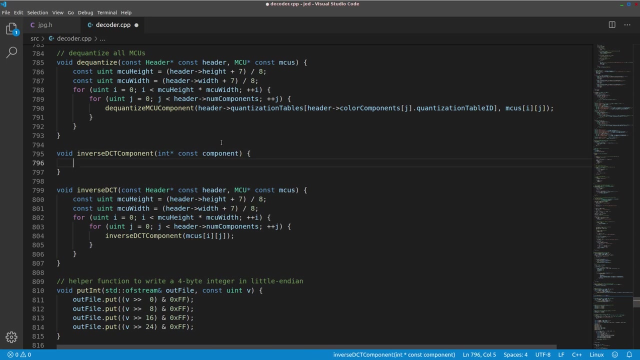 We'll perform inverse DCT on a component, so we need this inverse DCT component function And this is going to follow very closely with the pseudocode we just wrote. Like I said before, we want to store the result of all of the sums into a separate array. 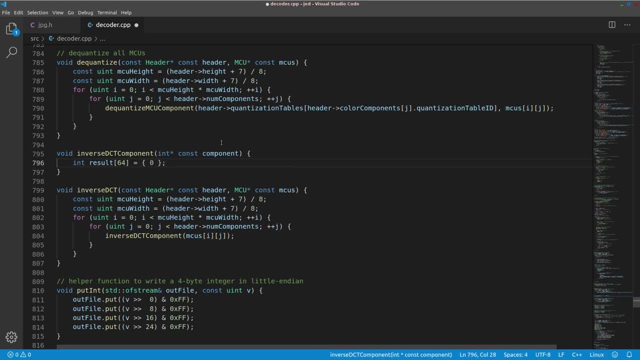 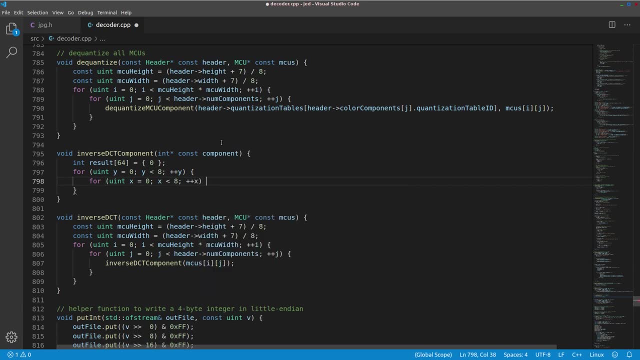 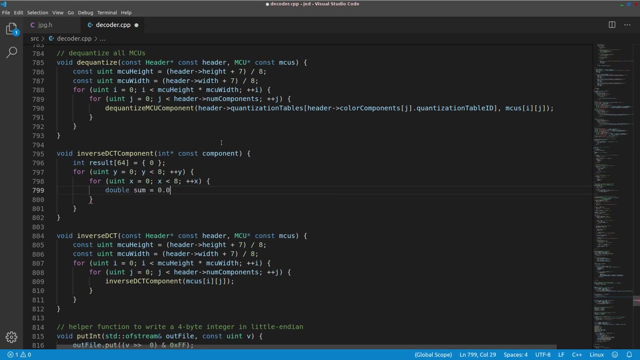 That way we don't overwrite the DCT coefficients as we compute. We want to loop for y and x For every pixel in the MCU. we want to calculate the sum And to do that we need to loop through all DCT coefficients. 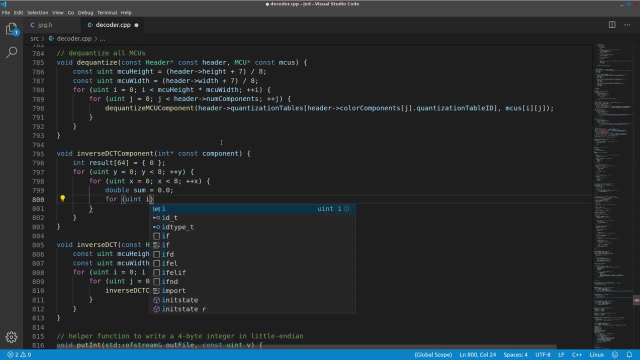 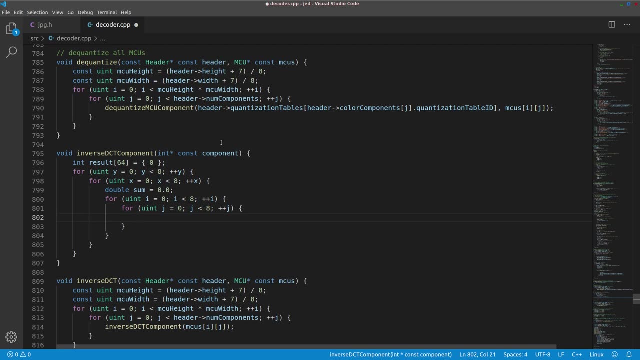 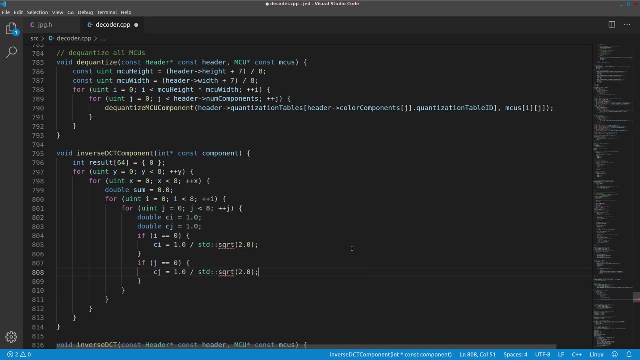 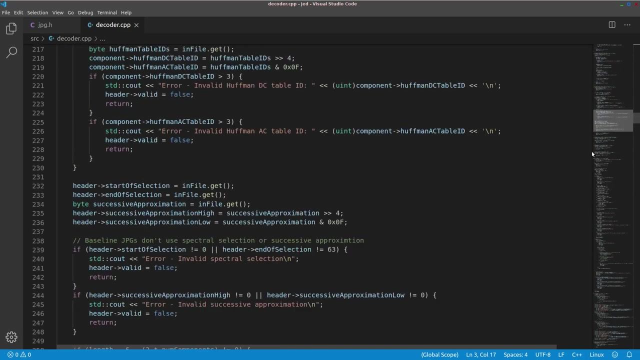 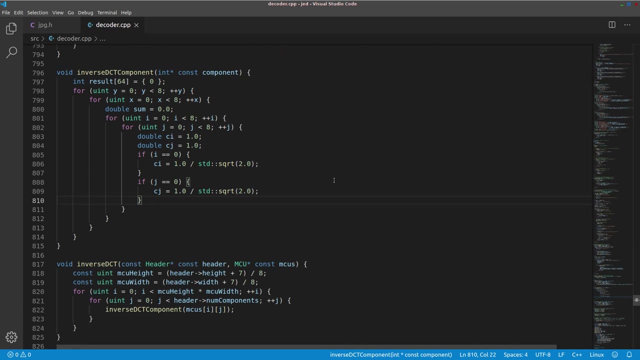 Hence i- j. We need to determine the values of c- i and c? j based on whether or not i and j are 0.. And to get square root we need to include c-math. Now we just need to add to sum based on x, y, i, j, ci and cj.